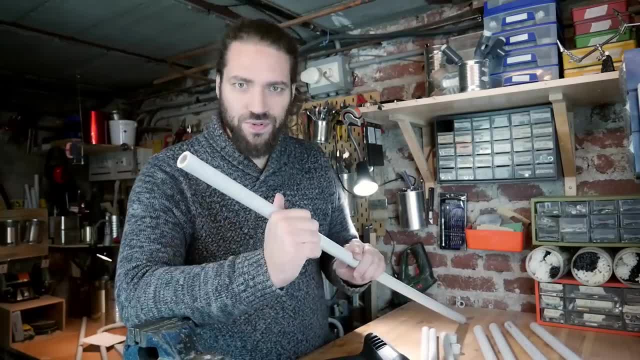 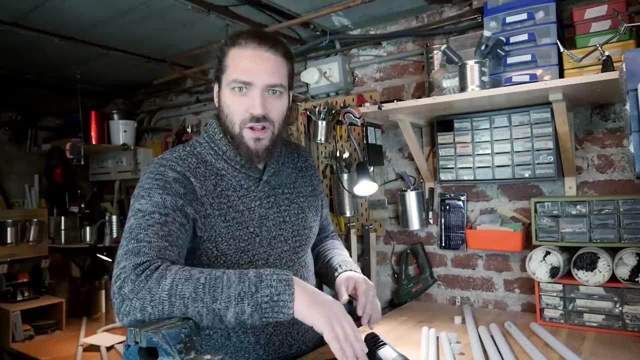 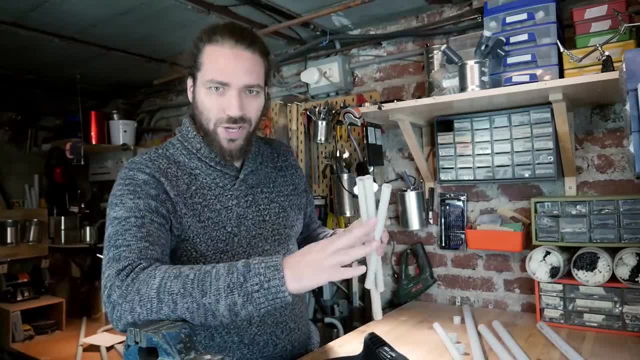 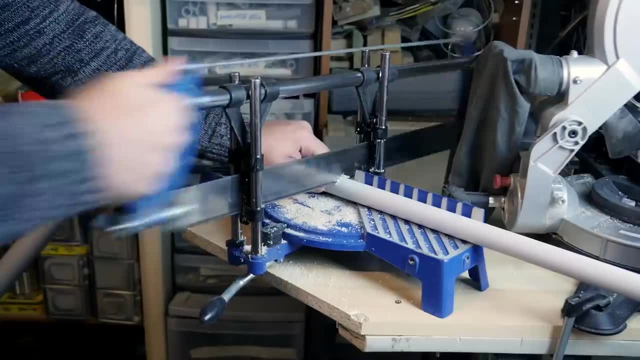 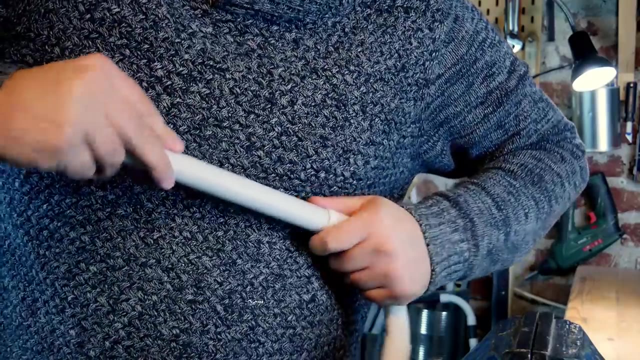 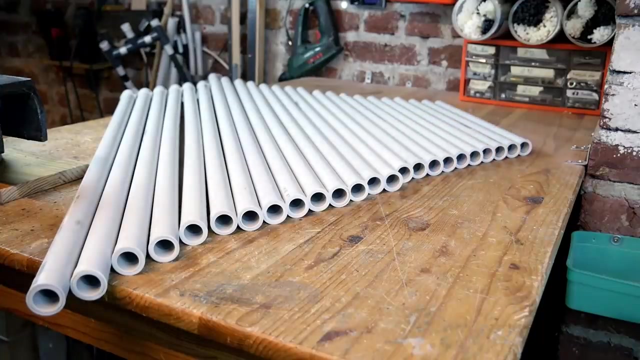 I made a low D sharp. I made a low D sharp. I made a low D sharp. Sounds okay to me, Let's go. 24 more pipes. I got my 68th notes. Before building the instrument structure, I want to sample it. 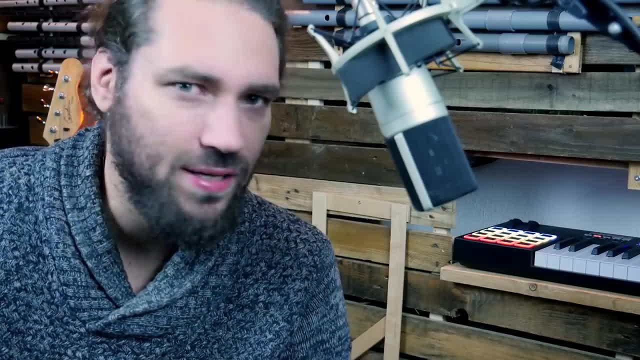 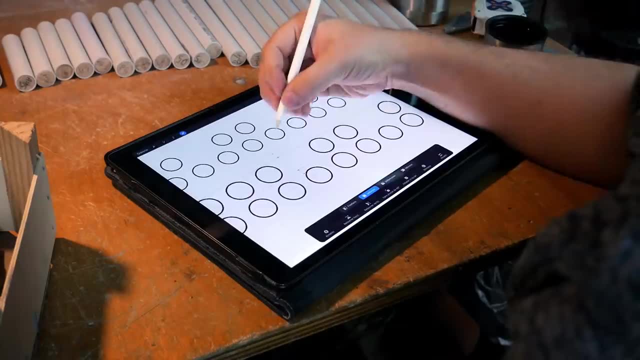 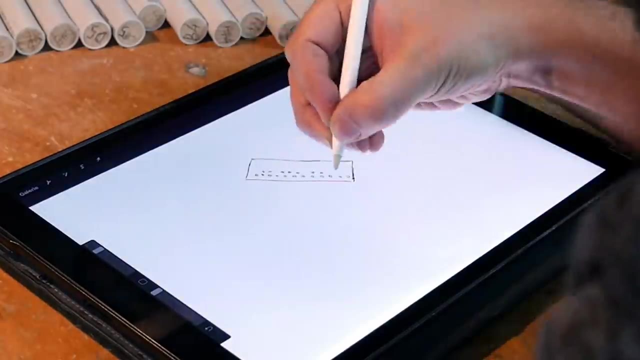 Done. My fingers hurt so much Stupid idea. Can't wait to play it on a keyboard. I don't want the instrument to be too big. It will be more a recording studio instrument than a live performance one. The keyboard will be in two ranges, disposed like piano keyboard. 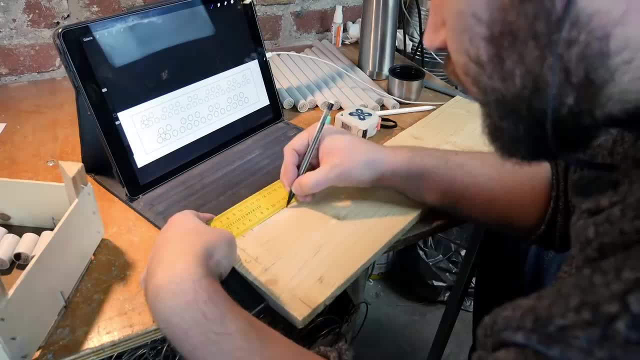 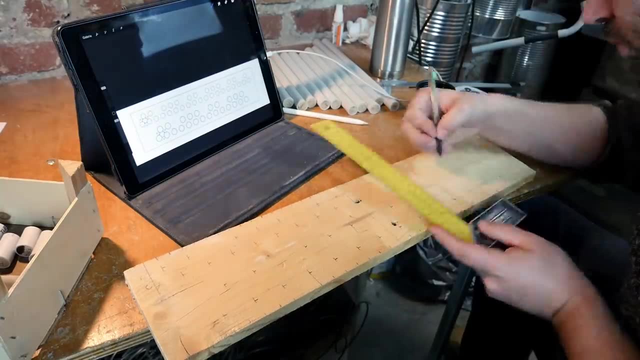 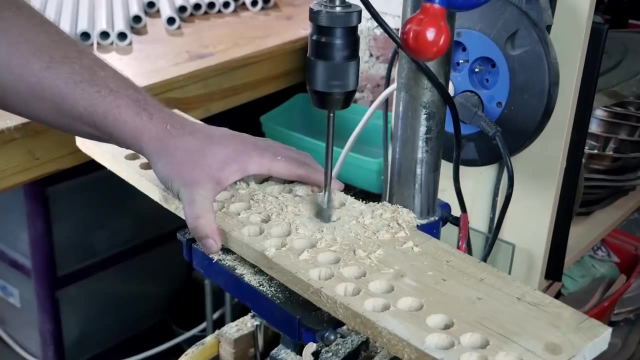 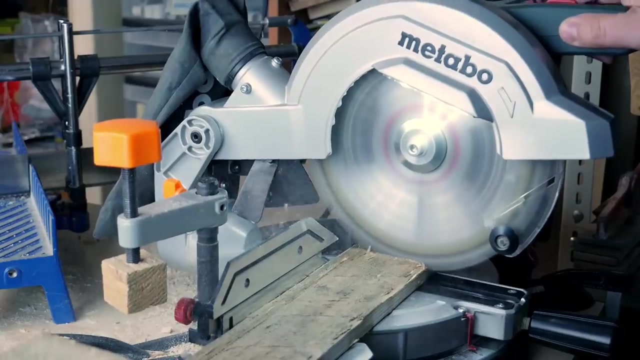 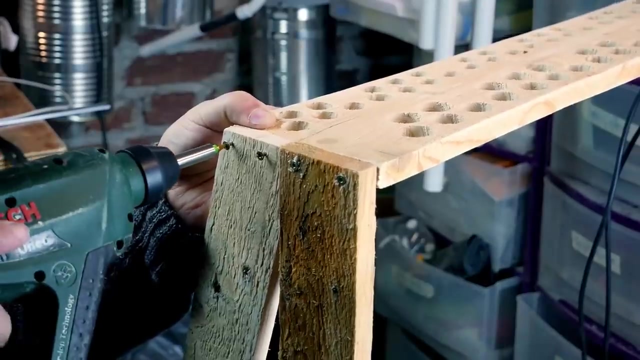 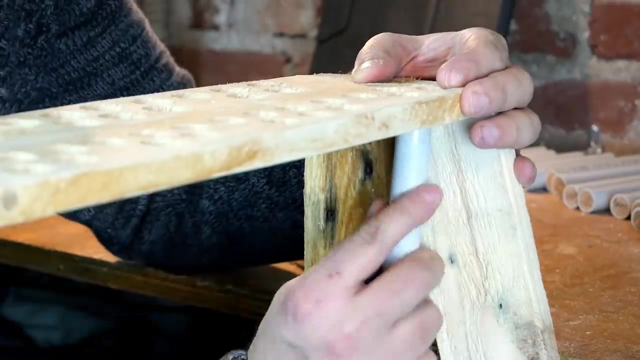 One range for the 20 millimeter diameter, One range for the 25 millimeter diameter. To hold the pipes, I just drill into a wood board. that will do it. To hold the pipes, I just drill into a wood board. that will do it. 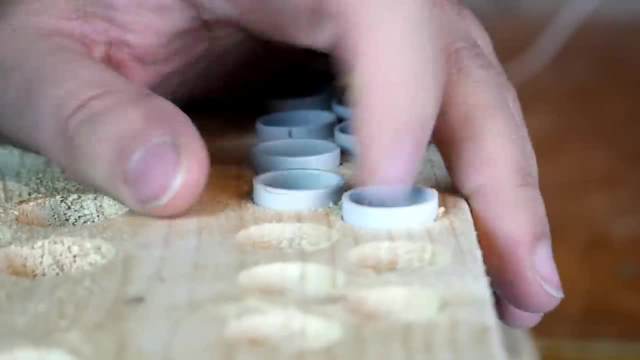 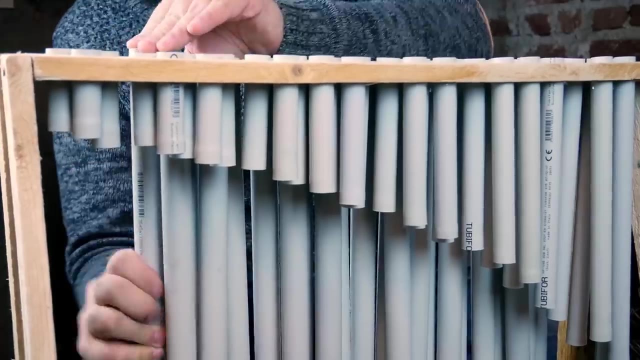 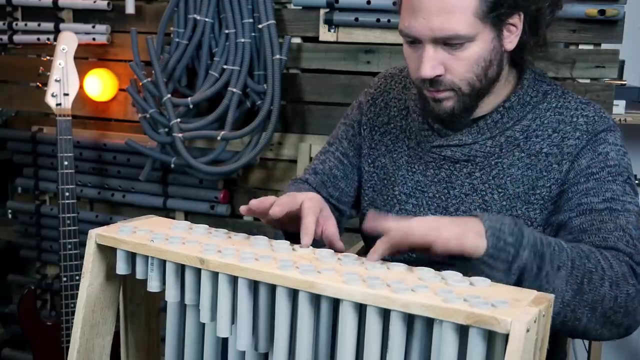 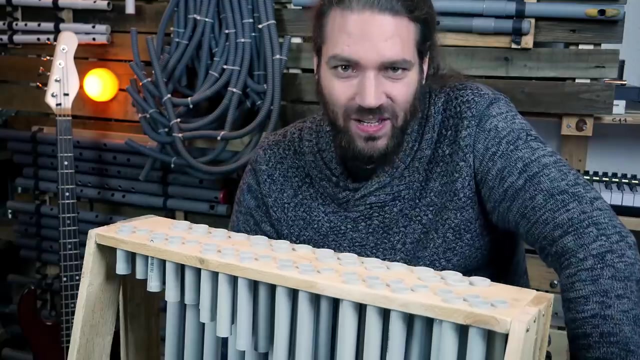 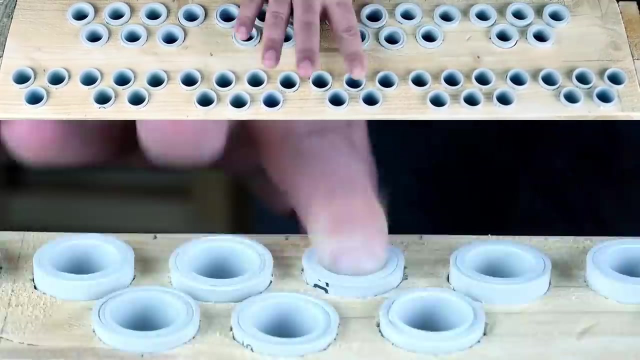 To hold the pipes I just drill into a wood board. that will do it. The instrument is down four octaves and a half. I see only one cover for a first track with this instrument. Now I have to chocolate My fingers hurt so much. 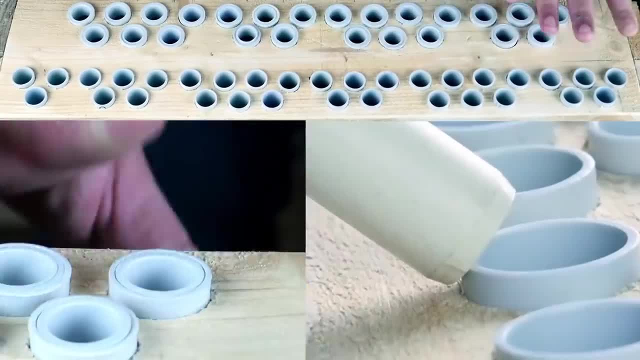 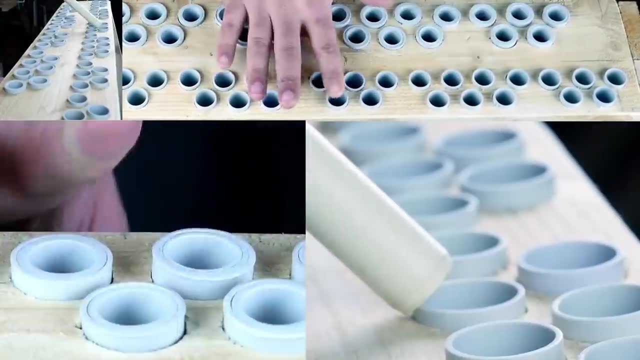 I don't want the instrument to be too big. I don't want the instrument to be too big. Let it be. I want it to be like a sick baby. Let it be. I got to love it. I got to love it.